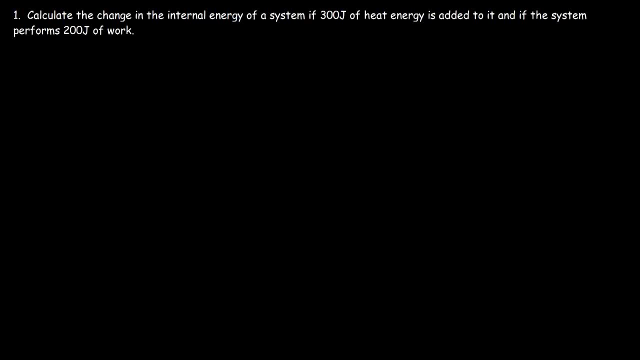 Let's work on this problem. Calculate the change in the internal energy of a system if 300 joules of heat energy is added to it and if the system performs 200 joules of work. Now, to get the answer, we need to use this formula. 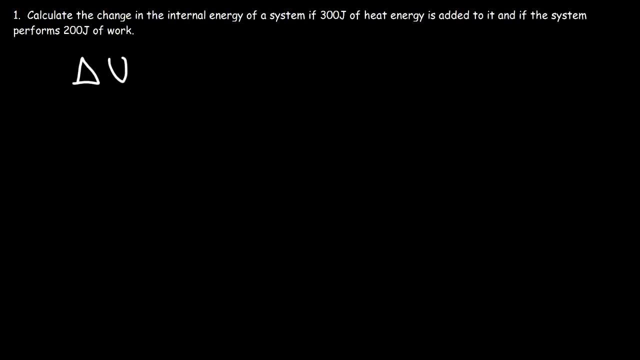 Delta. U, which represents the change in the internal energy of the system, is equal to Q, which represents the heat energy flowing into or out of the system, minus W the work performed by the system. Now this equation is associated with the first law of thermodynamics. 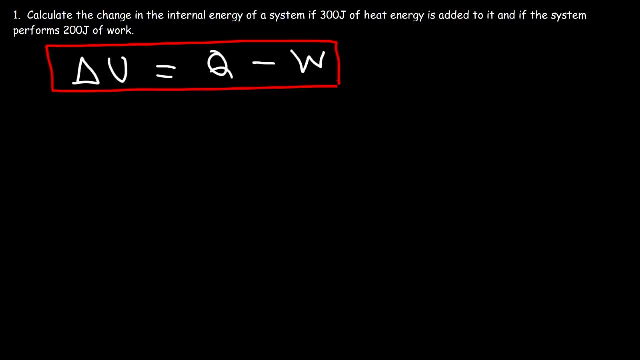 which basically is the principle of the conservation of energy. So in thermodynamics there's two ways in which heat, or rather there's two ways in which you can change the internal energy of a system. You can do work on it. 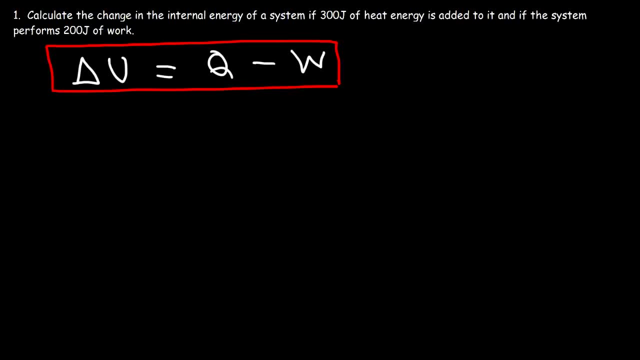 You can do work on a system, or the system can do work on the surroundings, or heat can flow into or out of a system, And so those are two principle ways in which to change the internal energy of a system in thermodynamics. 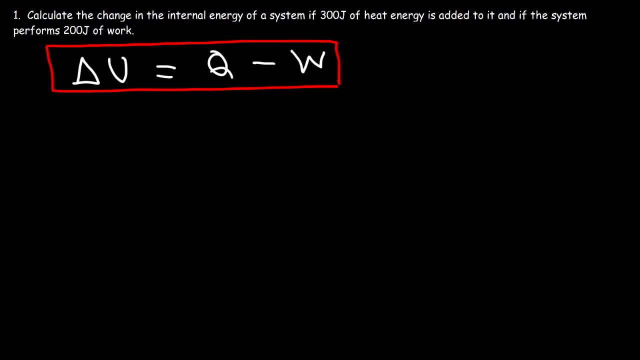 So energy has to be conserved. It can't just come from anywhere. Now you need to know that if Q is positive, heat energy is added to the system. If Q is negative, heat energy is removed from the system. Now, if W is positive, that means work is done by the system. 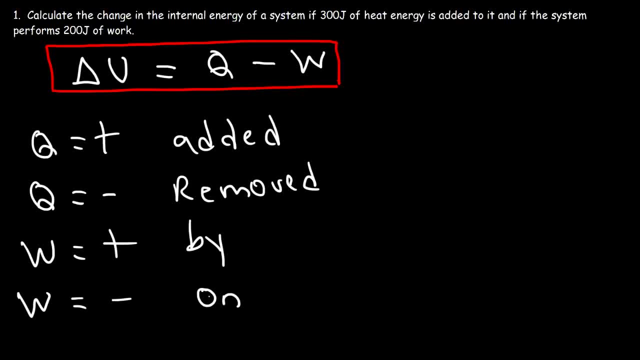 And if W is negative, work is done on a system. Now, these sign conventions are for physics. For chemistry it's opposite for work. In fact, in chemistry you'll see a positive sign as opposed to a negative sign, But in physics 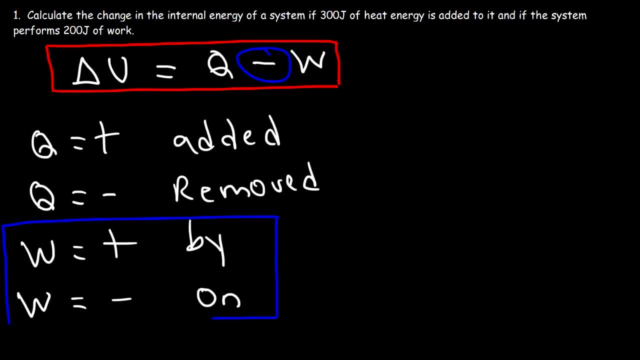 it's going to be negative, and these are the sign conventions for work when dealing with physics. Now let's go ahead and finish this problem. Now, what is Q and what is W? in this problem? Q is associated with heat energy, which is 300 joules. 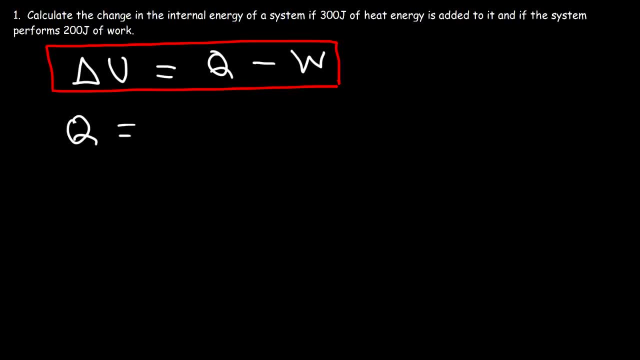 Is Q positive 300 or negative 300?? Now notice what it says. It says 300 joules of heat energy is added to the system. So that means Q is positive 300.. And then it says the system performs 200 joules of work. 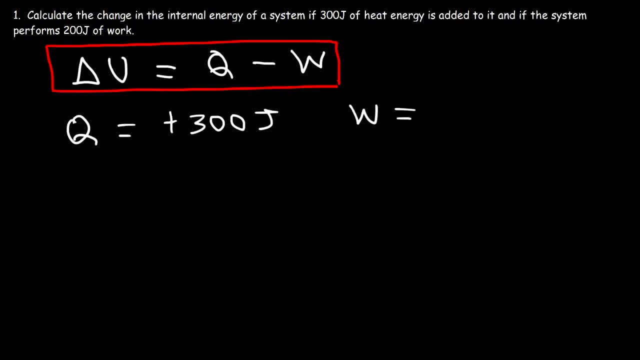 So work is done by the system. In physics that's going to be positive 200 joules. In chemistry that would be negative 200 joules. So now we can calculate the change in the internal energy of the system. 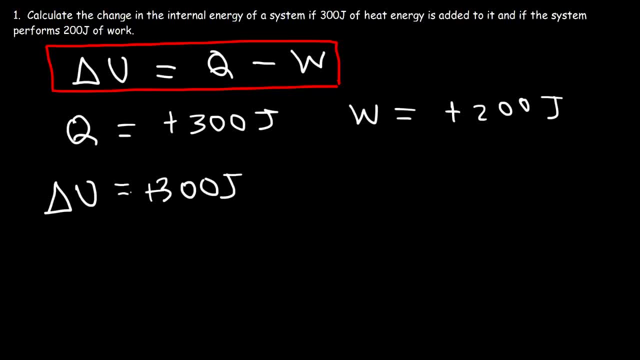 So it's going to be 300 joules. That's Q, It's positive, And then minus W, which is positive, 200 joules. So 300 minus 200.. So the internal energy of the system increases by 100 joules. 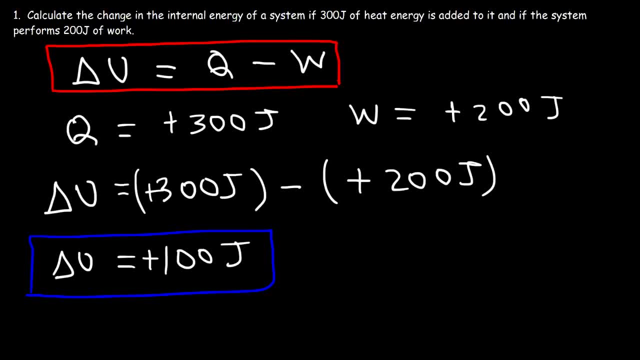 And that's the answer. And so, as you can see, for thermodynamics, there's two ways in which you can change the internal energy of the system. It's by transferring heat to it, That is, heat energy, Or by performing mechanics. 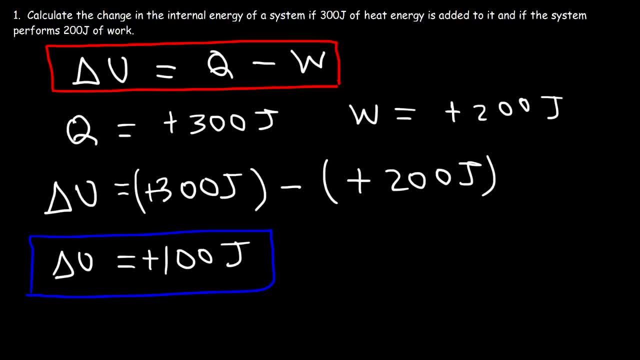 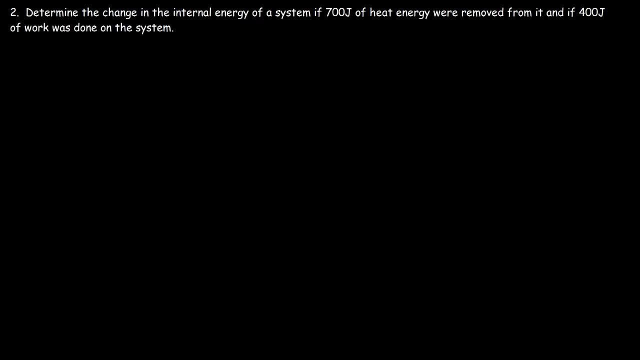 Mechanical work on a system. Now let's work on number two. Determine the change in the internal energy of a system if 700 joules of heat energy were removed from it and if 400 joules of work was done on a system. 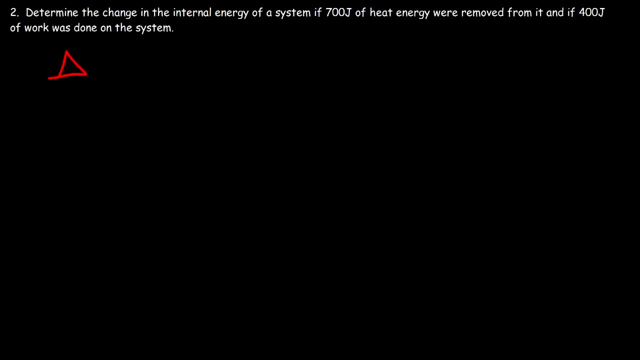 So go ahead and try this problem. Feel free to pause the video. So this is the main equation that we need to use, But first let's calculate Q and W. So 700 joules of heat energy was removed from the system. 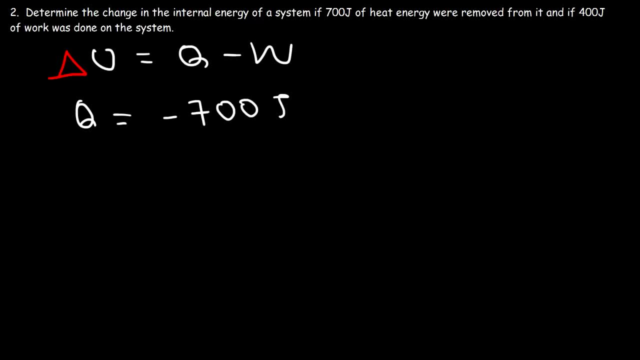 So therefore, Q is negative 700.. And W. we can see that 400 joules of work was done on a system. If work is done on a system, W is negative. So this is going to be negative 400 joules. 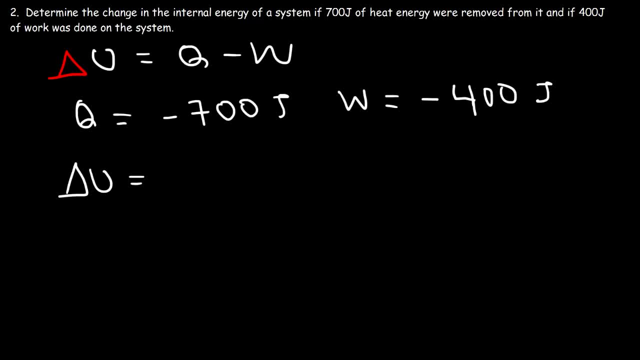 So now we can calculate the change And the internal energy of the system. So Q is negative 700. And W is negative 400. So this is going to be negative 700 plus 400. And so the internal energy of the system decreases by 300 joules. 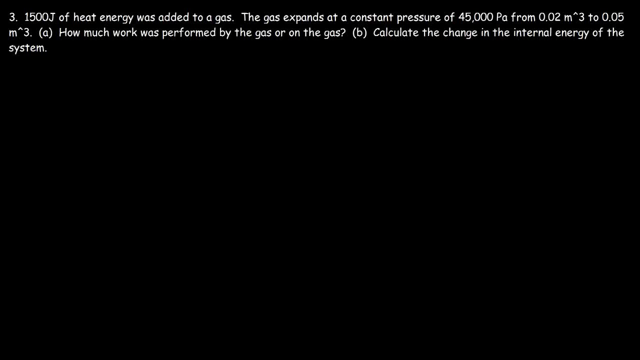 And therefore that is the answer Number three. If 400 joules of heat energy was added to a gas, the gas expands at a constant pressure of 45,000 pascals from 0.02 cubic meters to 0.05 cubic meters. 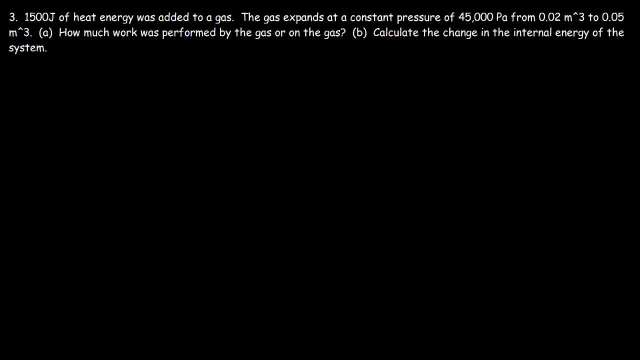 How much work was performed by the gas or on the gas. So to calculate the work performed by a gas if the pressure is constant, you could use this formula: Work equals P times delta V. Now you need to know that 1 pascal times 1 cubic meter is equal to a joule. 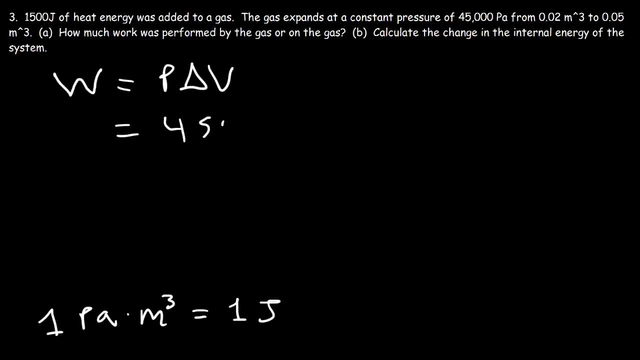 So we have the pressure in pascals- It's 45,000 pascals- And we have the volume changes in cubic meters, So we don't have to change the units. The final volume is 0.05 cubic meters. 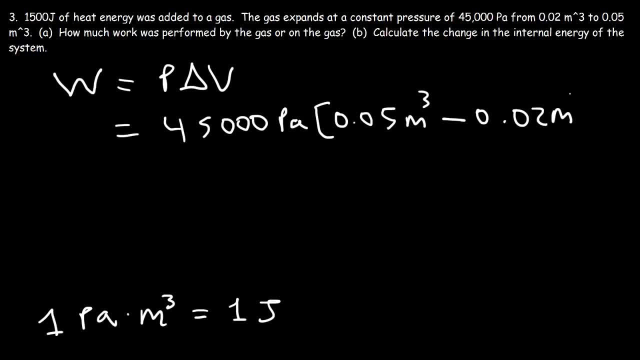 And the initial volume is 0.02 cubic meters. So it's going to be 45,000 pascals multiplied by a change in volume of positive 0.03 cubic meters, So the work is 1350 joules. 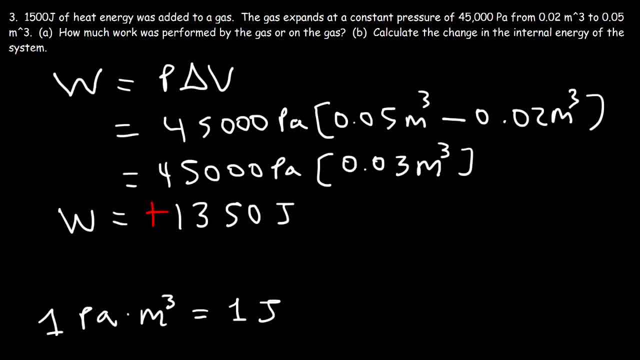 And it's positive. Since the work is positive, was the work performed on the gas or by the gas? Whenever W is positive, the work is performed by the system, So it's performed by the gas. Now, what else do we know in this problem? 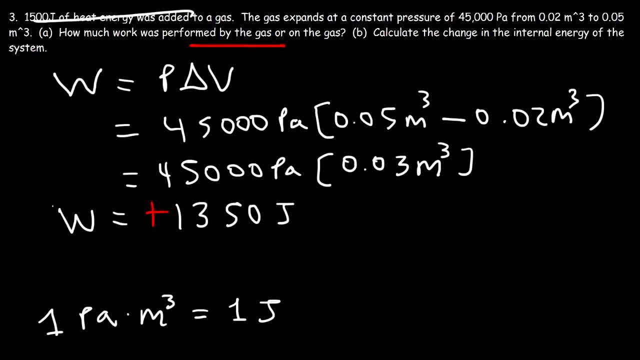 Now we know that 1500 joules of heat energy was added to the gas, So therefore Q is positive 1500 joules. So now we can move on to part B: Calculate the change in the internal energy of the system. 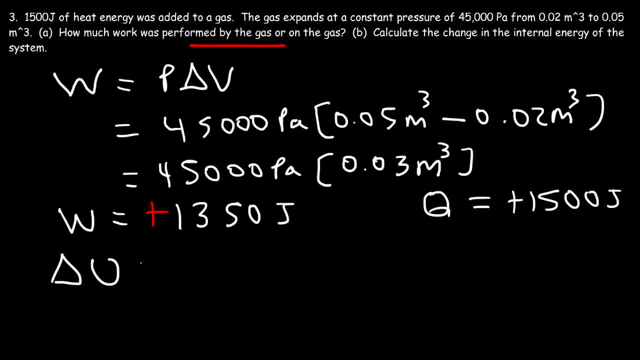 So we can use the same formula as last time. The change in internal energy is Q minus W. So Q in this example is positive 1500 minus W, which is positive 1350.. So it's 1500 minus 1350.. 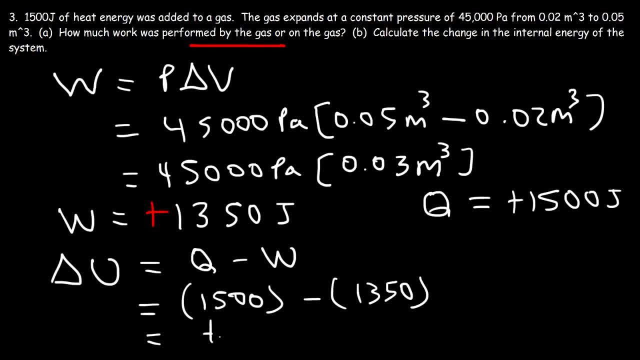 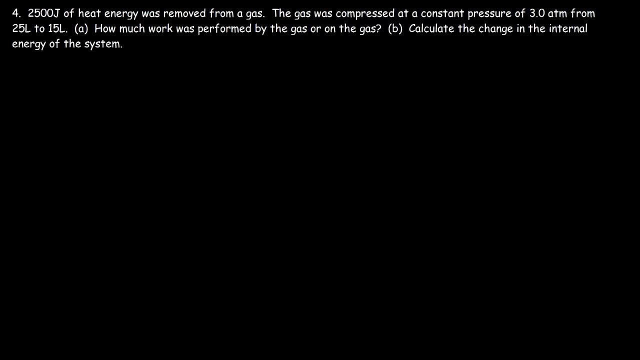 And so the internal energy increases by 150 joules. And so that's the answer in this problem for part B. Now let's move on to our last problem. You can try it if you want to. 2500 joules of heat energy was removed from a gas. 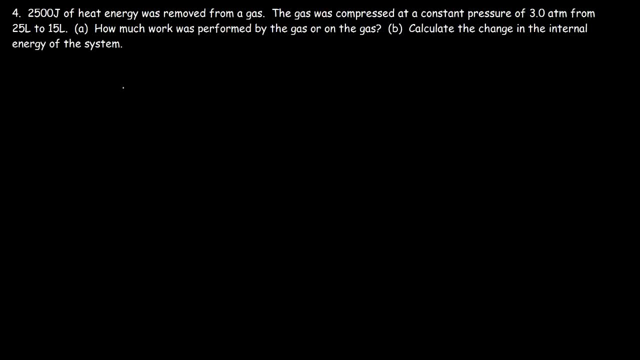 So if you want to pause the video and work on it, feel free. Now, because heat energy is removed from a gas, we know that Q is negative, So in this example it's negative 2500.. Now the gas was compressed at a constant pressure of 3500. 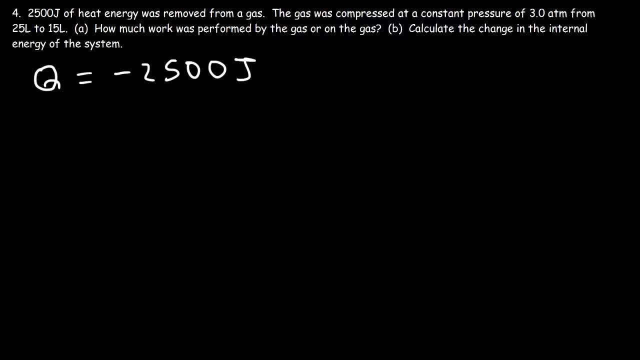 So we have 3 atm, from 25 liters to 15 liters. How much work was performed by the gas or on the gas? In the last example, the gas expanded And so work was performed by the system. In this case, the gas is being compressed. 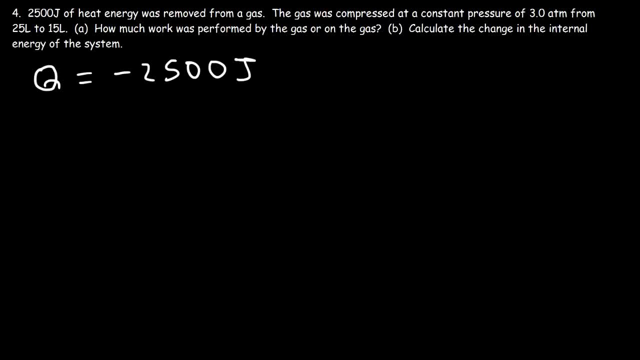 The volume is decreasing, So an outside force is needed to compress the gas. So in this example, work is being done on the gas, So we should expect a negative answer. Now the work is going to be the pressure times, the change in volume. 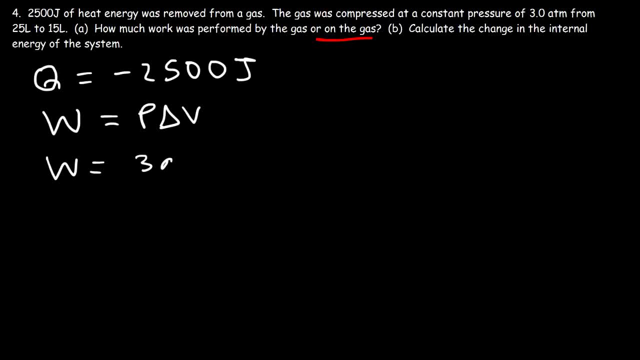 The pressure in this example is 3 atm And the volume, the final volume, is 15 liters minus the initial volume of 25 liters. So 15 minus 25, that's negative 10 times 3.. So this is going to be negative 30 liters times atm. 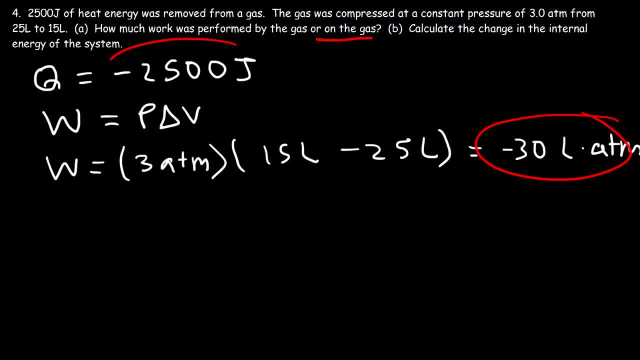 Now notice that we can't use this value along with joules because the units do not match. So we need to convert liters times atm into joules. So here's the conversion: 1 liter times 1 atm is equal to 101.3 joules. 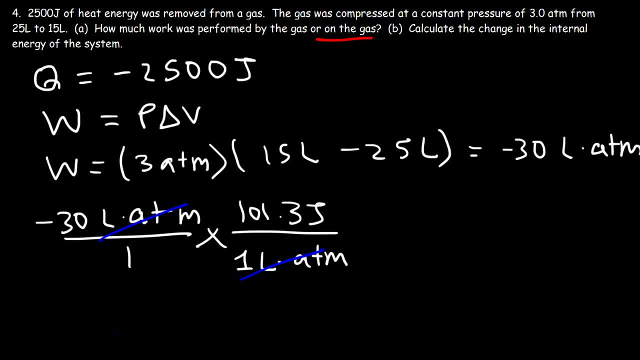 So negative 30 times 101.3.. That's equal to negative 3,039 joules. And because the work is negative, the work is done on the system as opposed to by the system. So now that we have Q and W, we can calculate the change in the internal energy of the system.